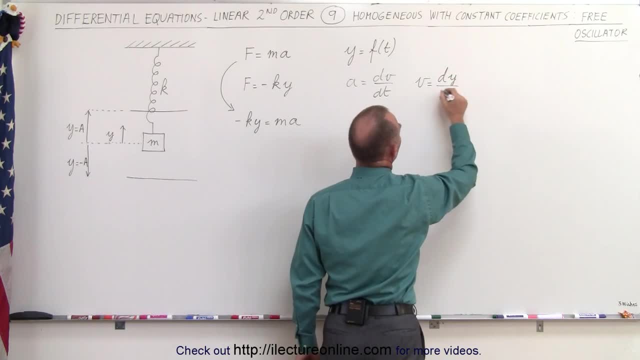 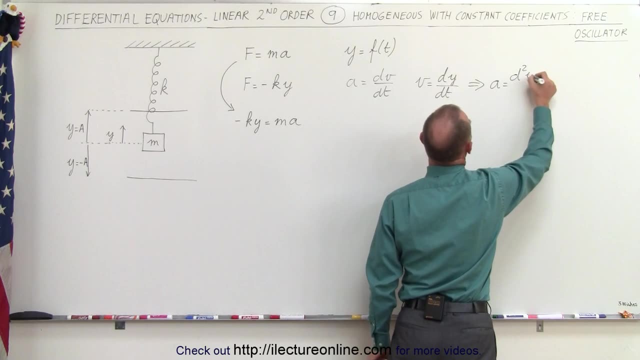 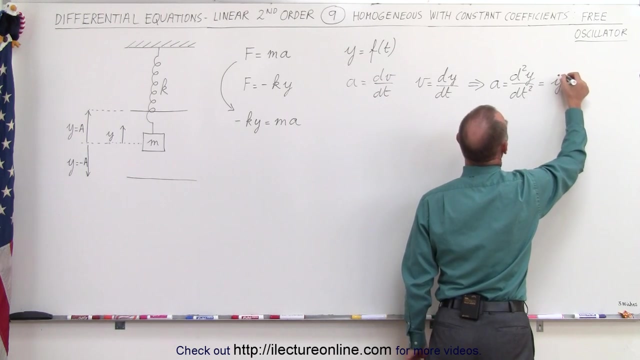 a parcel, i should use the d, the first derivative of the displacement rex with respect to time. this can then indicate that a is simply the second derivative of displacement with respect to time, and so this can be written as y double prime or even y double dot. so instead of using the prime symbol, we can use the dot symbol, because we realize now that 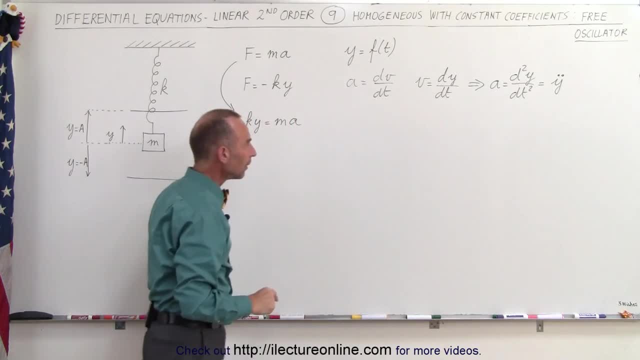 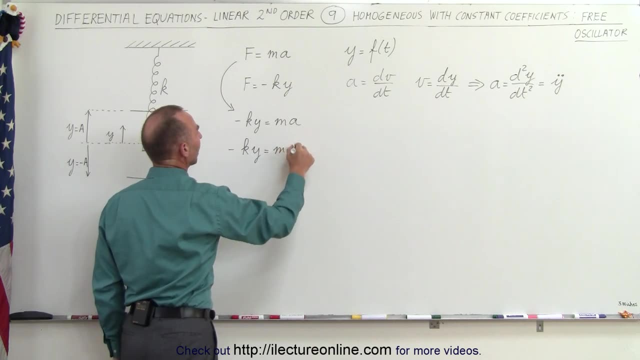 the displacement is a function of time, which means we can now write this equation as: minus k times y is equal to the mass times y double dot, because- and that's the same as y double prime- it's the second derivative of y with respect to time. that's why we use the double dot. 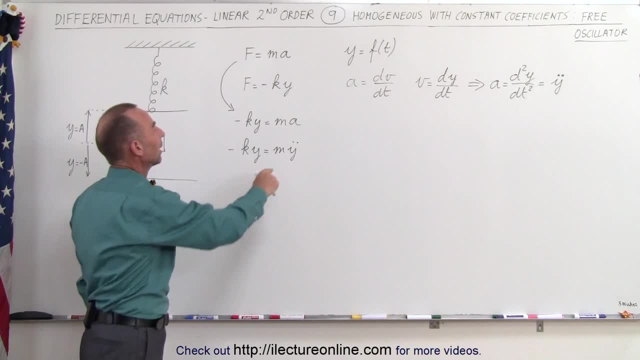 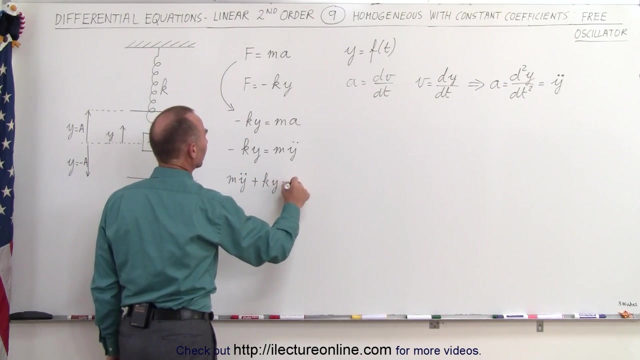 the notion notation here and that will then replace acceleration. if we now move everything over to one side of the equation and we have zero on the other side of the equation, this then becomes m times y, double dot plus k times y is equal to zero. i simply move this to the other side, becomes: 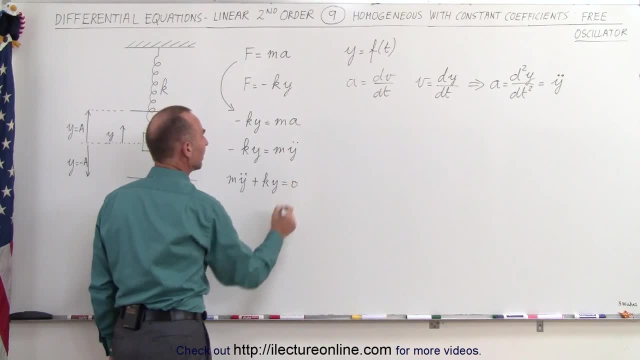 positive. flip the equation around and then i get this, and then finally, if i divide both side of the equation by m, i get y double dot plus k times y. double dot k over m times y is equal to zero, and this now becomes the form of a second order differential. 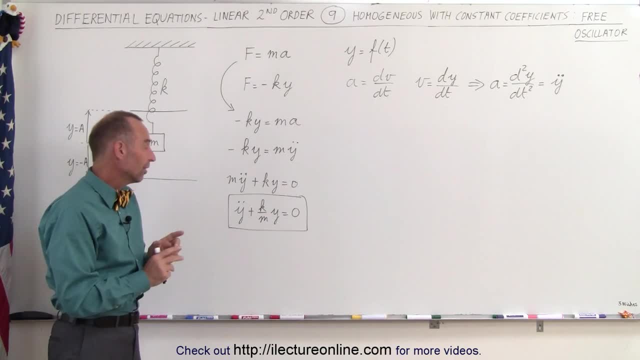 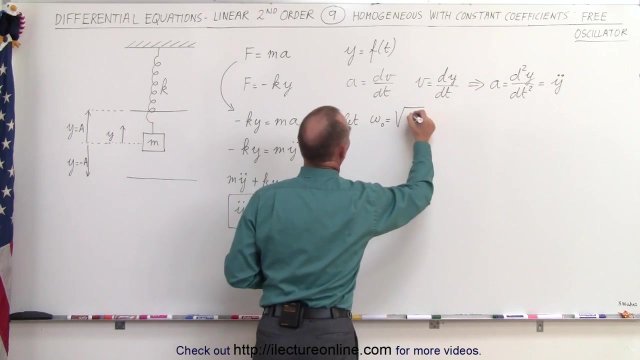 equation that is linear, that is homogeneous and that has constant coefficient, because k and m are both constant, so k divided by m would be a constant. to make things a little bit simpler, let's make a substitution. let omega sub naught equal the square root of k over m. when we do that, 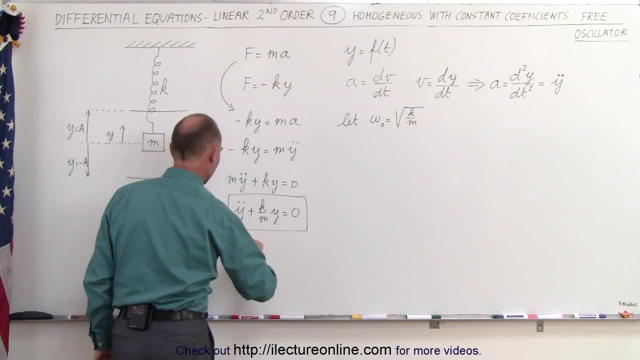 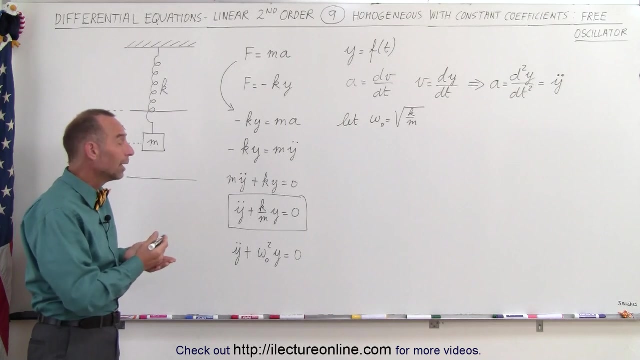 we can substitute that in here, so we can say that y double dot plus omega sub naught squared times y equals zero. but again, omega sub naught squared is simply another constant. now why did i make that substitution? well, from experience we know that when something oscillates back and forth there, 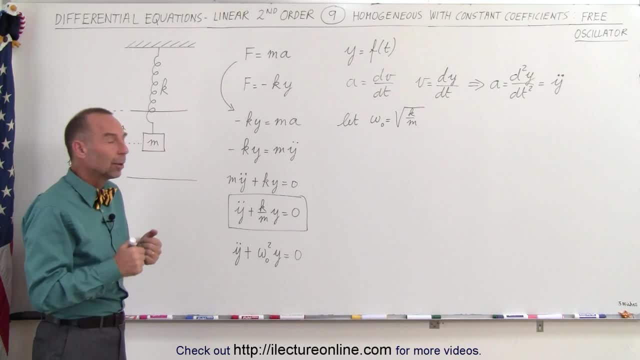 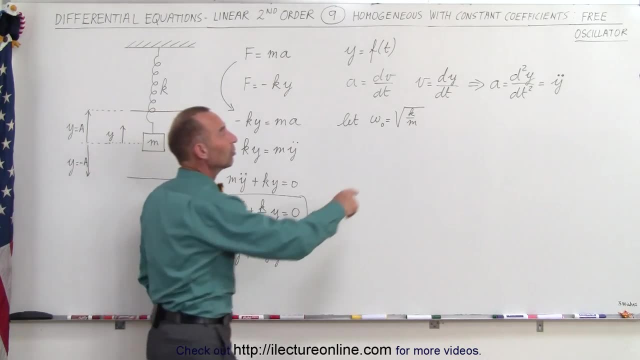 will be a certain frequency of oscillation, omega, and that would of course be the radial or the radian frequency, and that is always equal to the square root of k over m. if you make the spring stronger, we let k be bigger, then the oscillations will be more quickly. 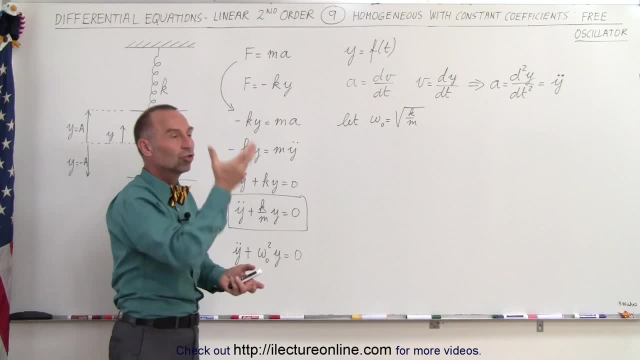 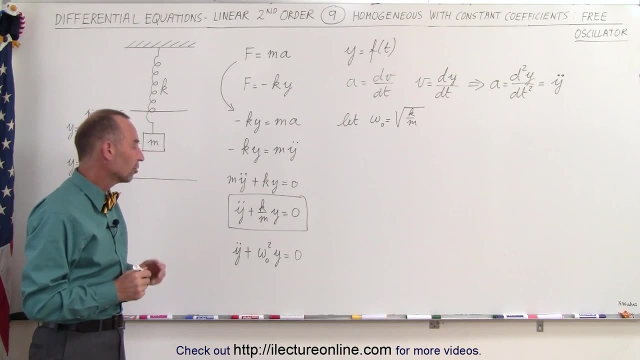 if you let n be bigger, then it takes longer for the mass to change, there's more inertia and the oscillations will be slower. so now, what is the general solution to this particular equation? remember that we learned in the previous video that the general solution, y, would be equal in. 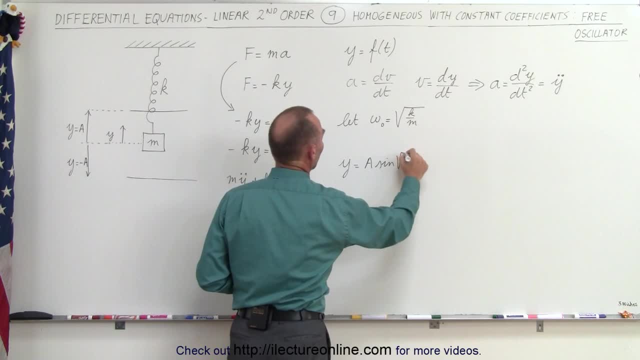 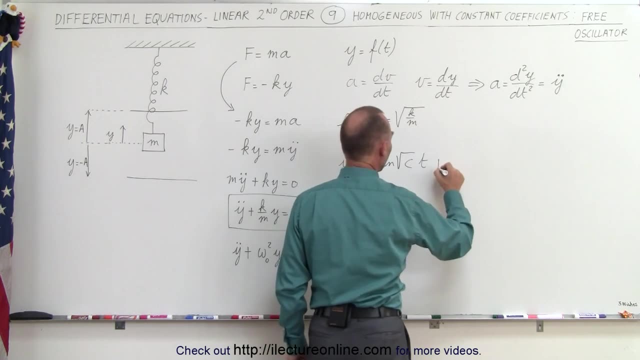 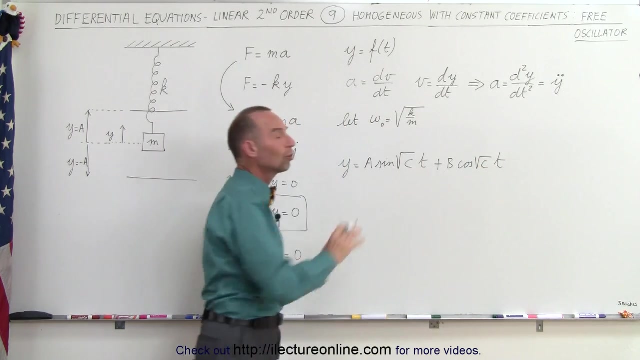 the form a times the sine of the square root of the constant, that is here times the variable. in this case the variable would be t plus b times the cosine of the square root of that constant times t. so that would be the general format of the equation. now, of course, in this case we know that. 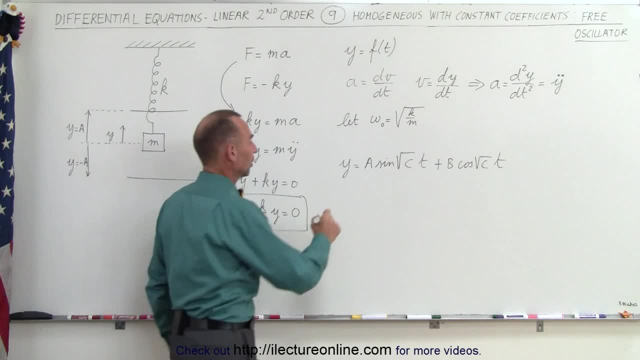 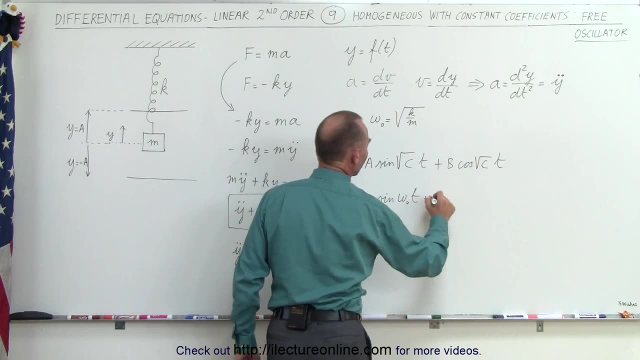 the square root of omega sub naught simply would be omega. so therefore we know that the solution would be: y is equal to the a times the sine of omega sub naught t, plus b times the cosine of omega sub naught t, and so this then: 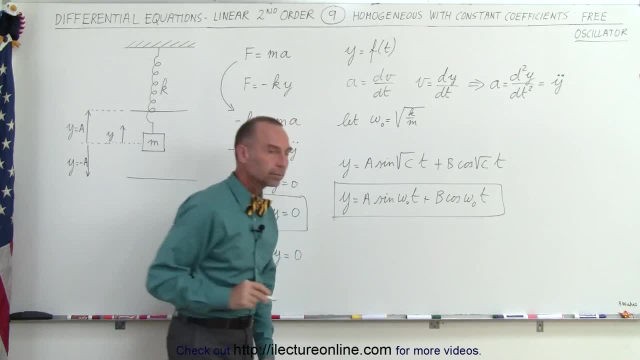 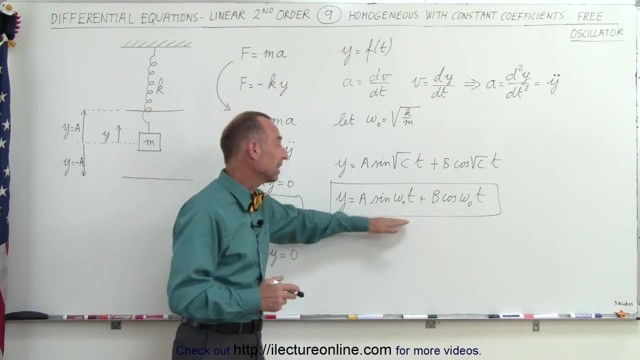 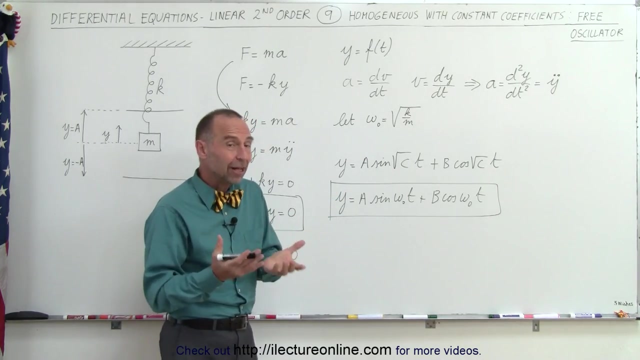 would be the general solution of the differential equation, so we shouldn't necessarily have to use both the sine and the cosine in the general solution. it would be sufficient to use either the sine or the cosine with the phase angle, and the phase angle would then be used to indicate. 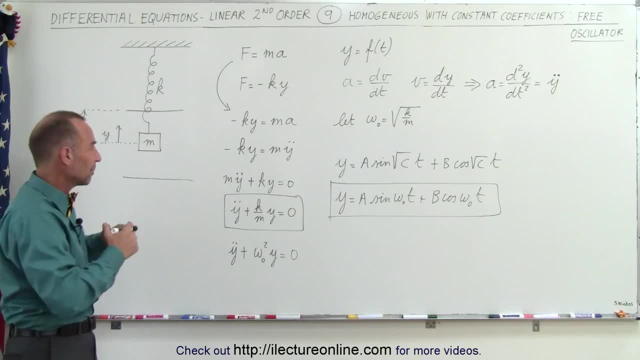 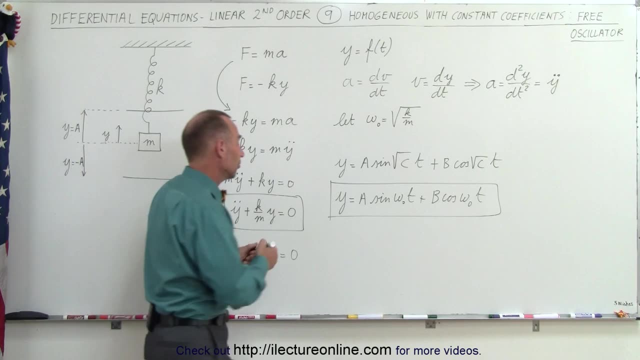 the initial condition now in our example right here, since we're just talking about the general solution, we don't have any initial conditions yet. we'll look at that at a later video. but here we can then say that it would be sufficient to say that the sine of omega sub naught t is equal to: 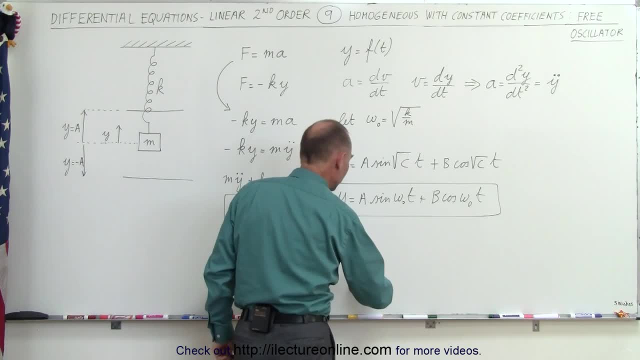 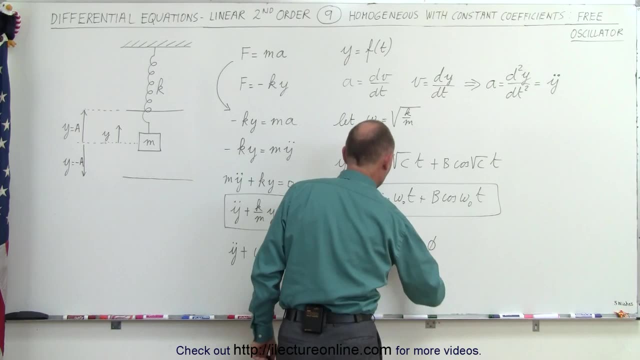 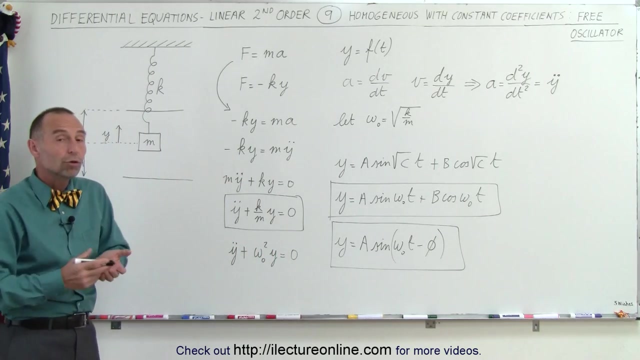 say that y can be written as a. the amplitude of the oscillation times, the sine of omega sub naught t plus or minus some phase angle. let's write as minus some phase angle, and this would then be the solution to the free oscillator. so we can you do, we could have used the cosine we could have used. 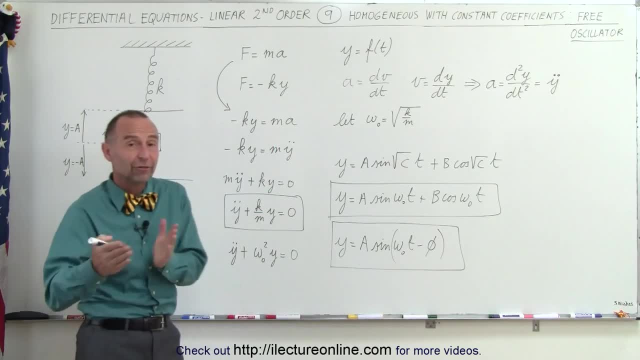 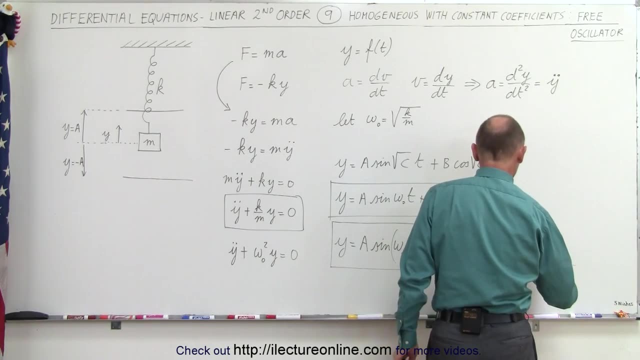 the sine. remember that the phase angle will then take care of the difference between the sine and the cosine. the only difference between the sine and the cosine is that they start at the different five degrees. so those speeches are different and there's a difference between the sine and the. 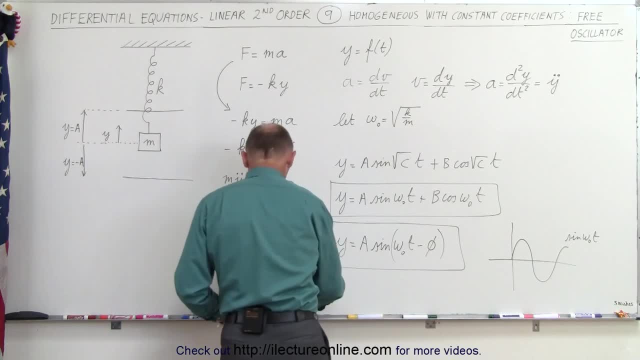 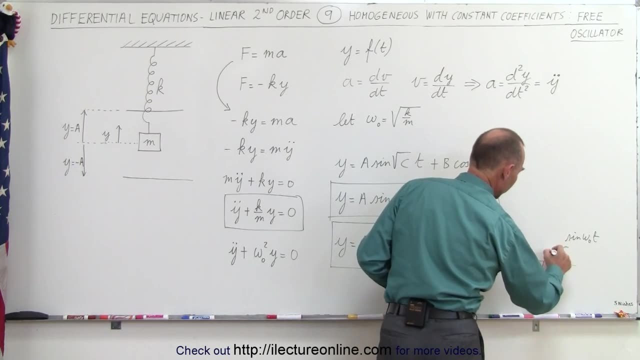 sine, so this would be the sine of the function. so this is what we call the sine of omega some, not t, and using a different color. the cosine starts here and then would look something like this: so it can- oop, it doesn't quite would go so high like that. so know that the cosine and sine there's.